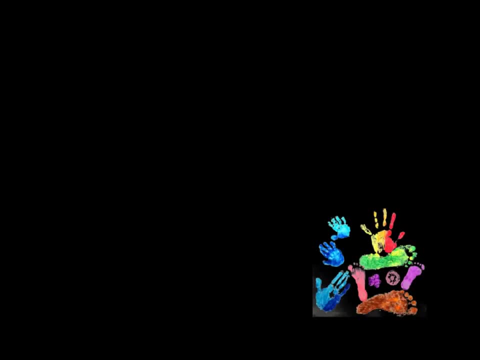 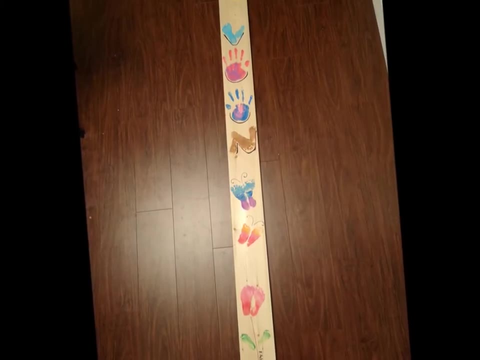 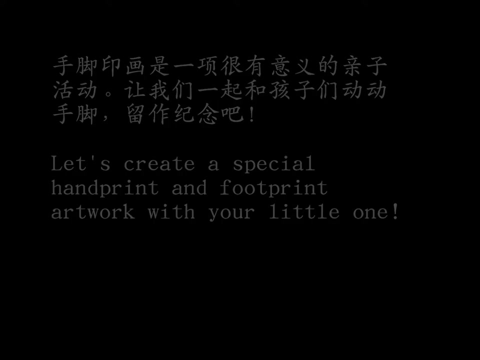 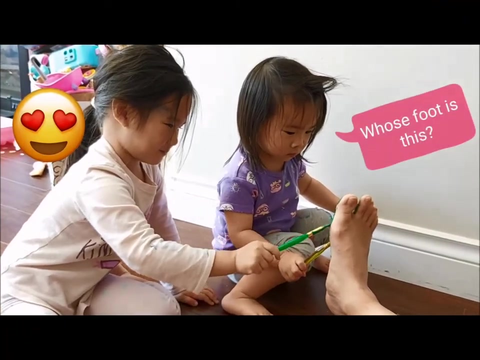 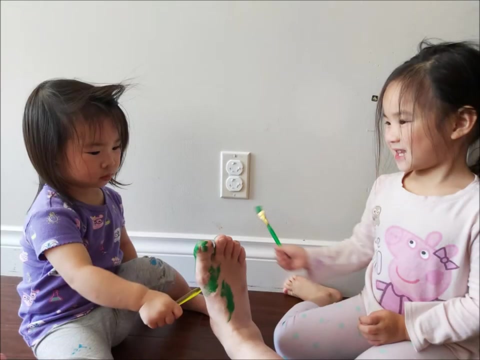 Make pictures and art. let's create. Pens, pencils, charcoal and paint: Make pictures, me and you. Stamps, glitter and glue: Make pictures and art. let's create. I love using all the paints. they're so nice. 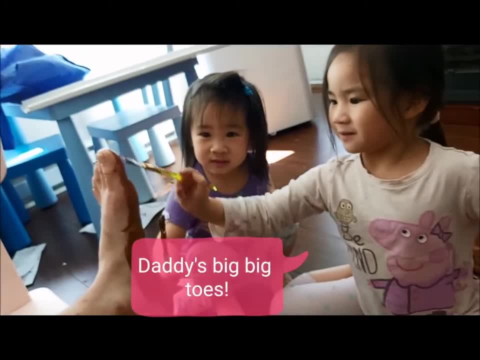 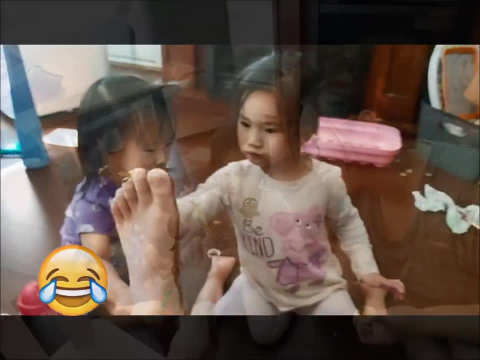 All the colors in the tray. they're so bright, Like my own rainbow to use. I've got greens, reds and blues. I love using all the paints. they're so nice For some messy fun. I love to take some glue. 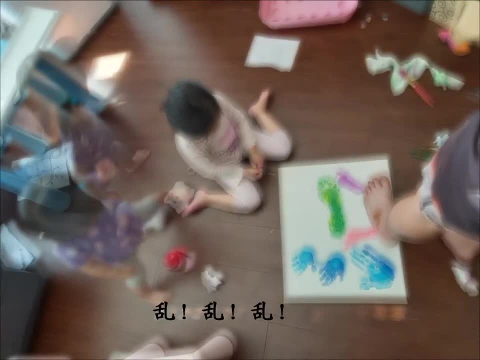 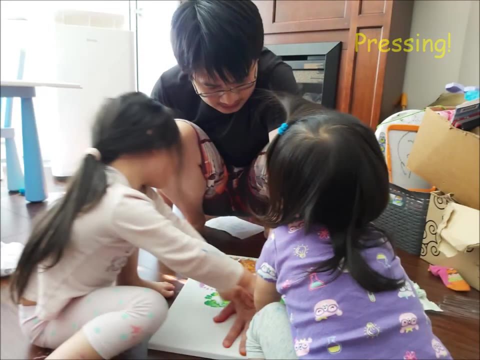 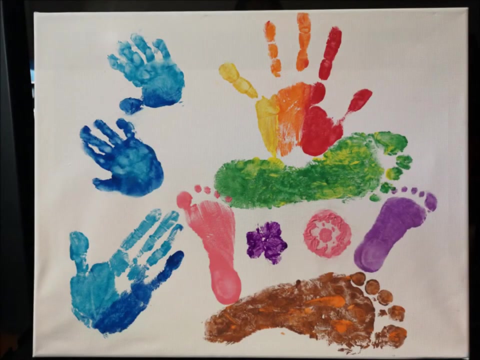 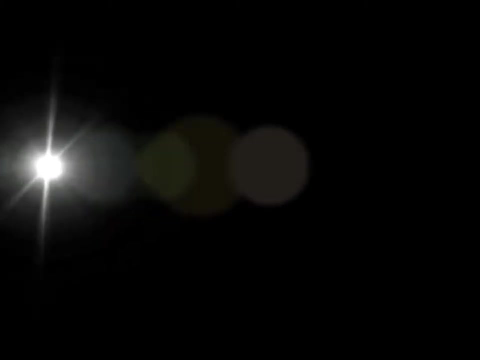 Add some glitter paper and some stars- Stamps too. Look at what I just made. I feel happy and amazed For some messy fun. I love to take some glue, Make pictures and art. let's create Pens, pencils, charcoal and paint. 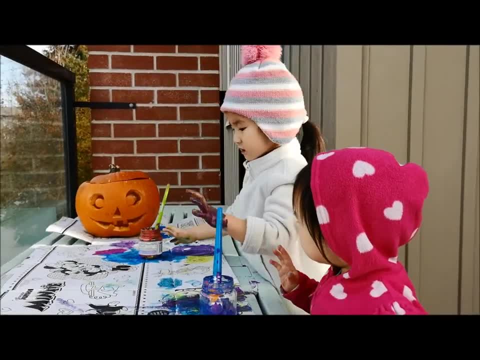 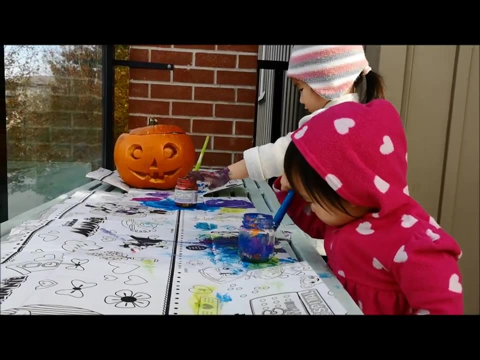 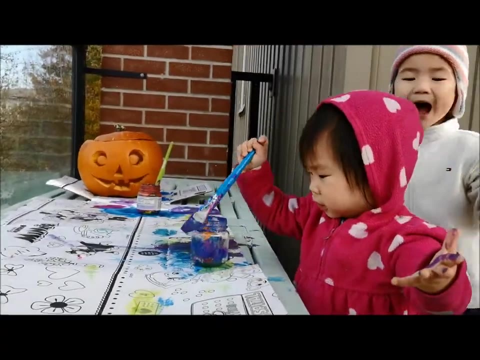 Make pictures- me and you. Stamps, glitter and glue. Make pictures: Stamps, glitter and glue. I love using all the paints. they're so nice. All the colors in the tray. they're so bright, Like my own rainbow to use. I've got greens, reds and blues. 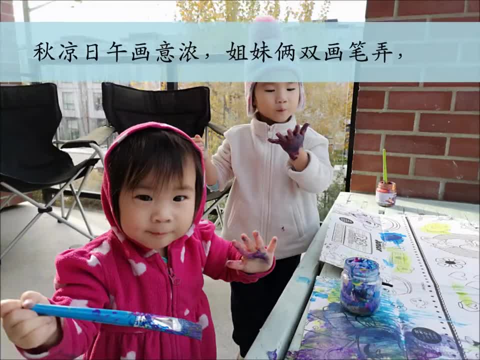 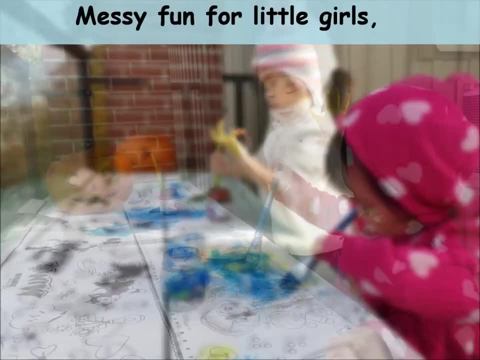 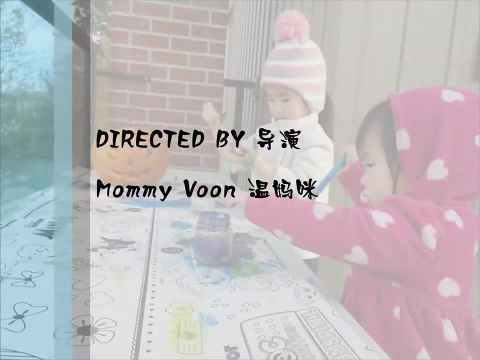 I love using all the paints. they're so nice. For some messy fun. I love to take some glue, Add some glitter paper and some stamps too. Make pictures and art. let's create. Look at what I just made. I feel happy and amazed. For some messy fun. I love to take some clue.